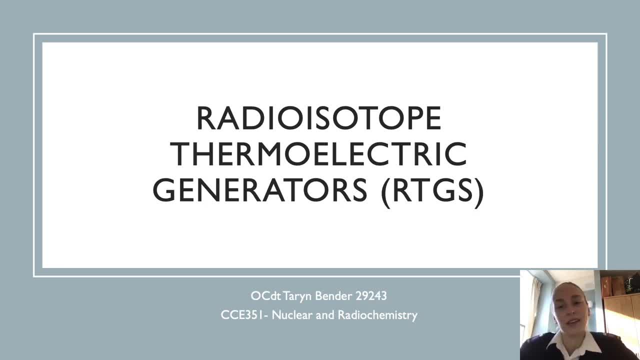 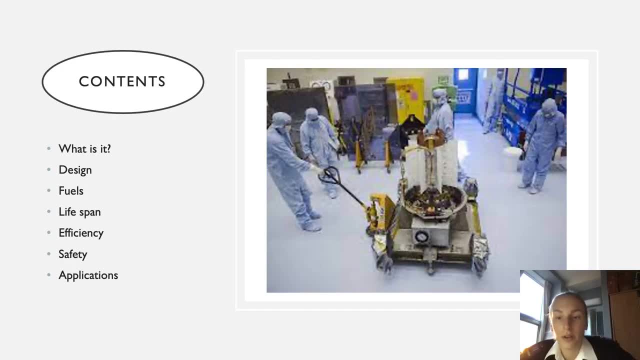 Hello and welcome class. My name is Taryn and I will be leading you through my presentation on radioisotope thermoelectric generators. First I will be going over the contents of my presentation, so after listening to me talk, you'll hopefully have a deeper understanding of what an RTG is. 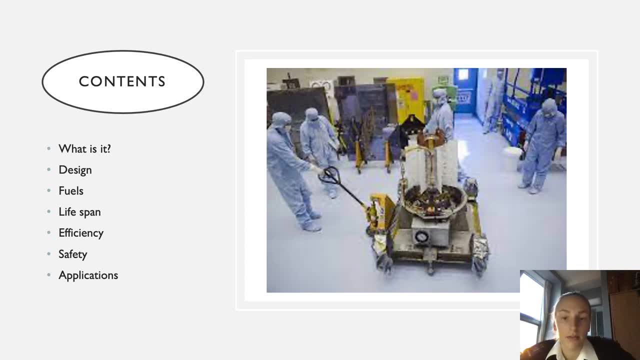 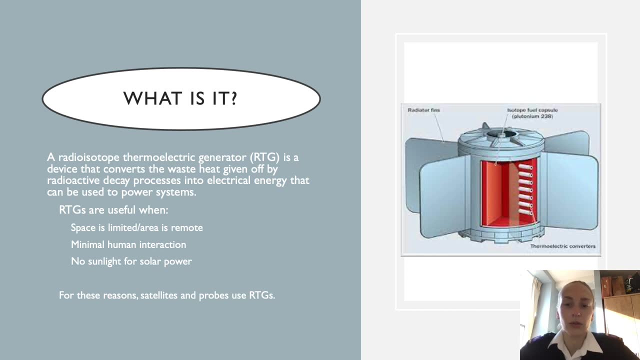 the design, the fuels used, the lifespan, the efficiency, any safety considerations and its applications. RTGs are devices that convert the waste heat given off by radioactive decay processes into usable electrical energy. This type of generator has no moving parts, So the first thing that I thought when I looked this up is: okay, that sounds really complicated. 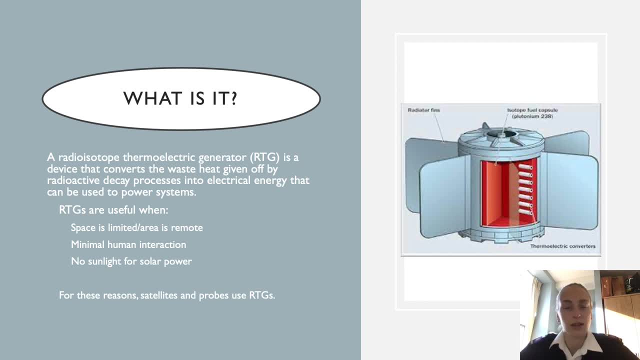 and, more importantly, costly. So why would somebody use this instead of other methods? RTGs are often installed in space-bound objects and remote structures or machines that cannot obtain energy efficiently by any other means. These devices are designed to be able to generate energy efficiently by any other means. 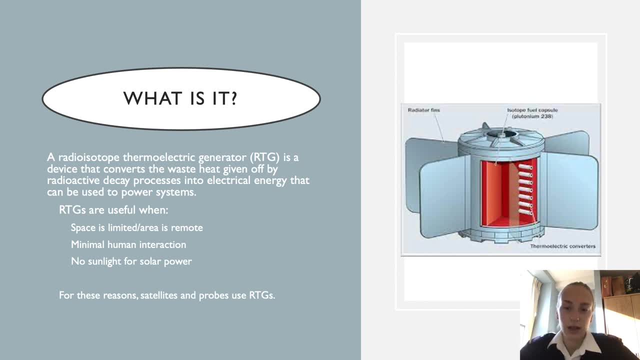 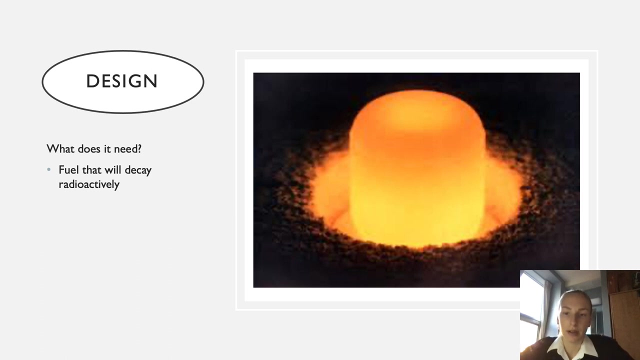 These include satellites, probes and even remote lighthouses. In this way RTGs are more efficient because the object being powered is not often accessible for human maintenance or direct sunlight for solar power. So an RTG needs fuel in the form of radioactive isotope that will decay. 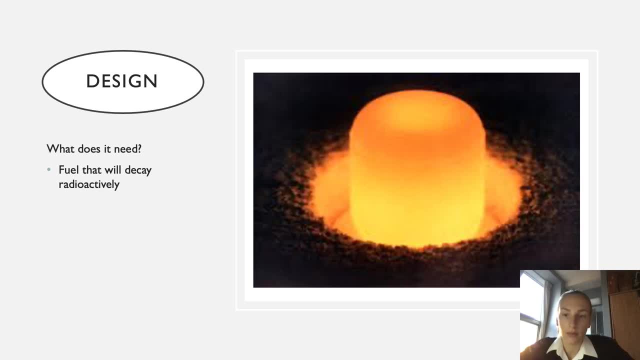 radioactively, But it won't just take any fuel, and we'll talk about that in a later slide. An isotope fuel pellet begins to decay radioactively once placed in an RTG, creating heat, and then, when it's decommissioned, it will decrease the rate of the reaction in the explosions. 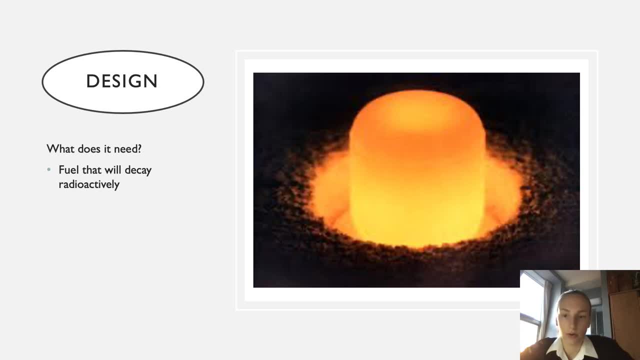 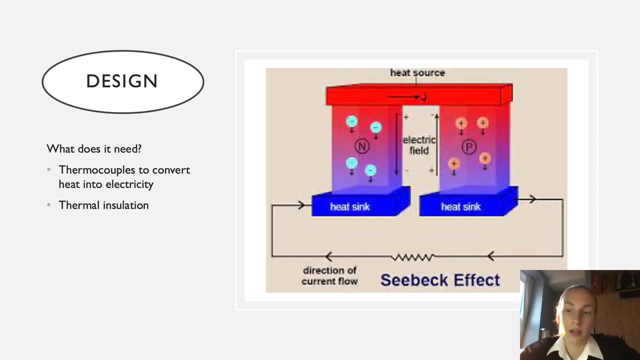 This causes the atmosphere to change and determine how the energy is being produced, then collected by heat distribution blocks, And here- this photo- we see a radioactive isotope fuel pellet- RTGs also need thermocouples to convert heat into electricity. These blocks that collected heat from the isotope 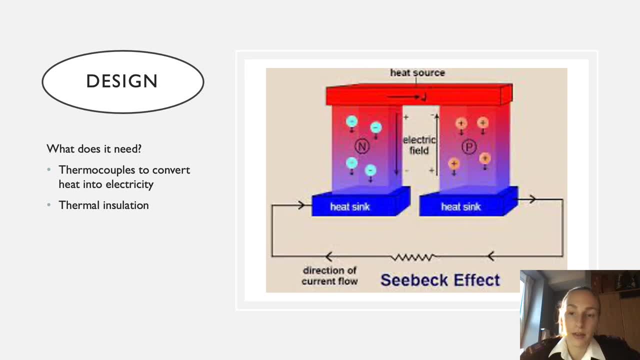 sends heat to thermocouples. Thermocouples rely on the Seebeck effect. The Seebeck effect demonstrates that when a differential in temperature is achieved, an electric voltage can be harnessed. This is very useful in RTGs as a strong temperature gradient. 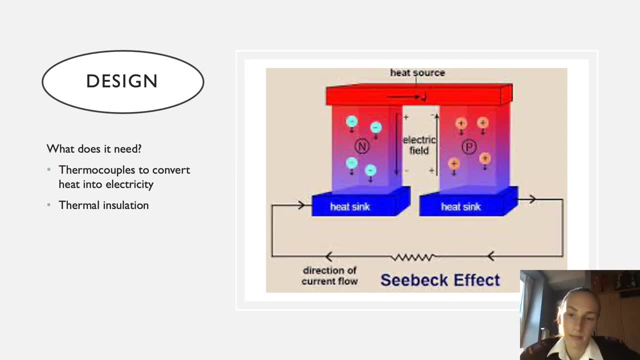 can induce a voltage difference that can, in turn, create an electrical current. This typically requires the use of materials with low thermal conductivity, which would allow for a wide range of temperature difference to accumulate between two ends, and high electrical conductivity, so that currents can easily flow. 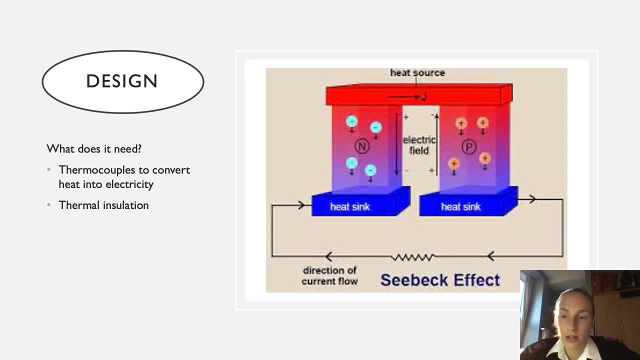 The last main component of an RTG is insulation. An RTG must be able to maintain that temperature gradient that induces a voltage difference. For this reason, RTGs are covered in layers of insulation with a hard outer shell to protect the inner workings of the device. 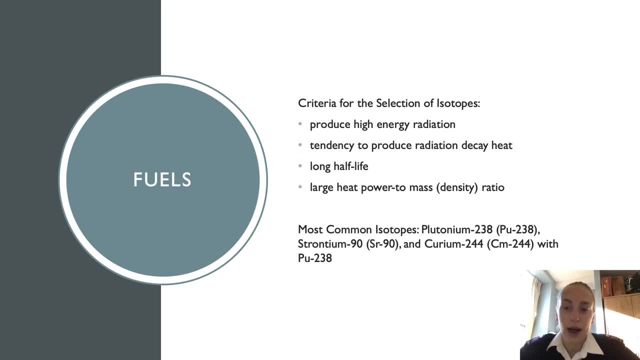 We know that an RTG needs fuel that will decay radioactively, but it does not just take any random fuel on the periodic table. The isotope pellet used must have the ability to produce high energy radiation- a tendency to produce radiation decay heat. 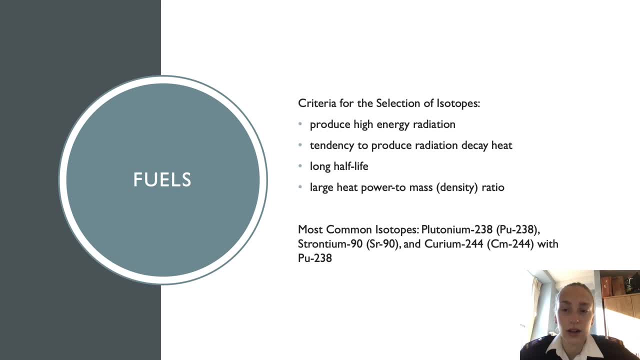 and have a long half-life for continuous energy production and a large heat to power mass or density ratio. Of the 1300 radioactive isotopes investigated by Dr Bertram C Blanc of Mound Laboratories in 1960, only 47 of these were found to have these characteristics. 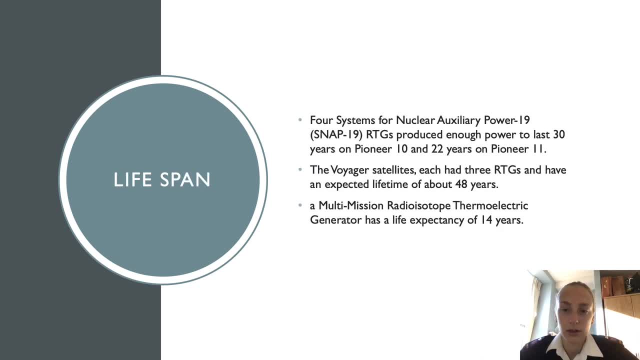 and even less can actually be used efficiently in an RTG. The main differences between RTGs and fissioned reactors are weight, lifetime and power output. The first Soviet topaz reactors in 1971 were capable of producing five kilowatt of electrical power. 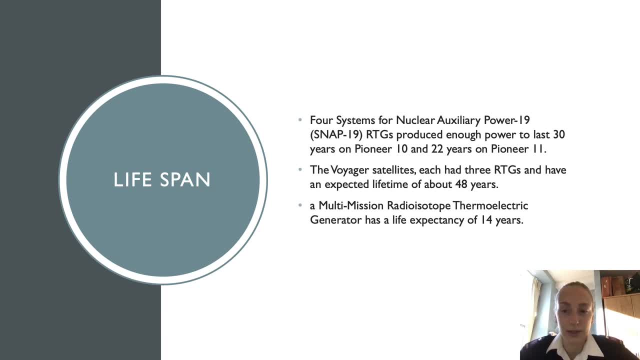 for three to five years and weighed 320 kilograms. Around the same time, a Systems for Nuclear Auxiliary Power 19,, or the SNAT-19 RTG, weighed only 14 kilograms and had an additional power output of about 40 watts. 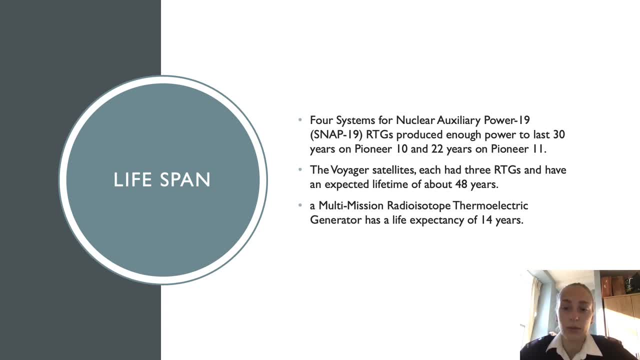 Four of these together produced enough power to last 30 years on Pioneer 10 and 22 years on Pioneer 11.. The Voyager satellites which launched in 1977, were each equipped with three RTGs, providing them with 470 watts of power. 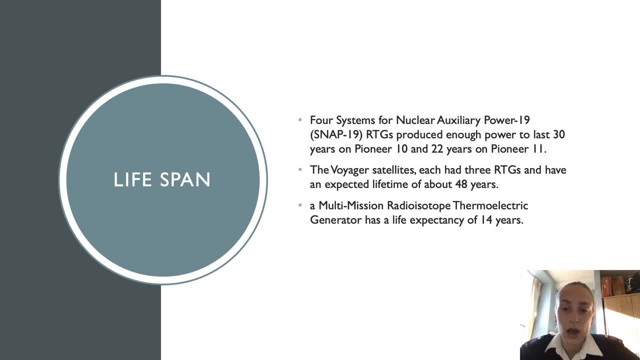 with an expected lifetime of power of about 30 watts. The Voyager has a lifetime of about 48 years, Currently a multi-mission radioisotope thermoelectric generator which is the RTG on the Curiosity rover on its own. 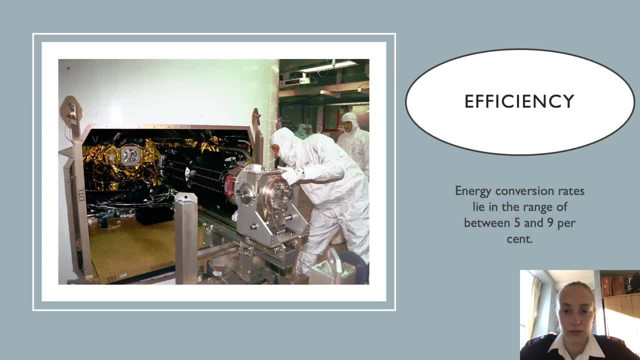 has a life expectancy of about 14 years. RTGs, though very reliable and long-lasting, are not overly efficient. Standard RTGs have an energy conversion efficiency of five to nine percent. Efficiencies above 10% have never been achieved in an RTG. Scientists have found that the efficiency of RTGs, which is the energy conversion efficiency of five to nine percent, has never been achieved in an RTG. Scientists have found that the efficiency of RTGs, which is the energy conversion efficiency of five to nine percent, has never been achieved in an RTG. 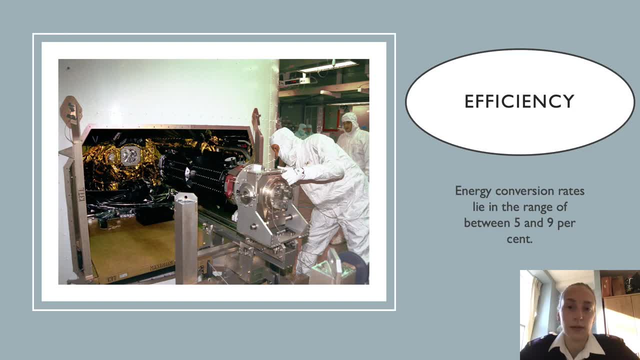 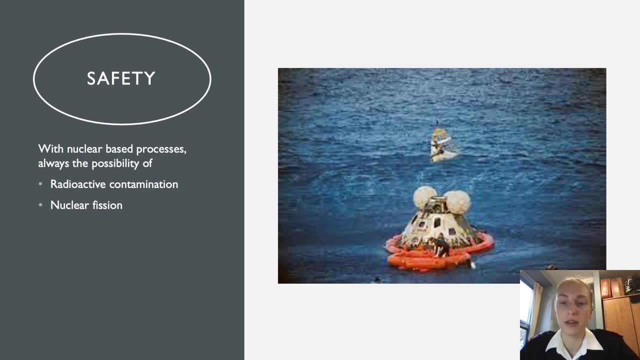 Scientists are still working to create more efficient and compact RTGs to this day. Scientists are still working to create more efficient and compact RTGs to this day. Having any nuclear-based processes in functioning devices always creates concern over human safety and possible radioactive contamination involved. 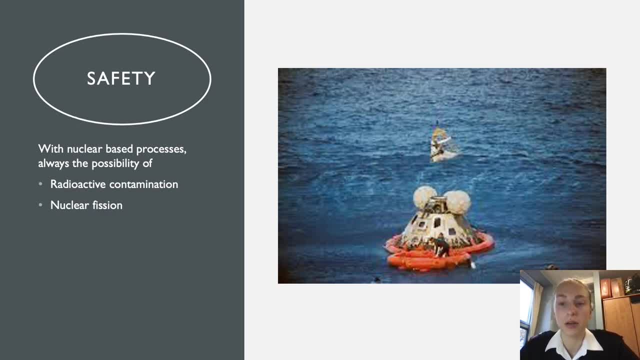 Even though RTGs are designed to function in remote environments where human populations are sparse or nonexistent. these questions are not unwarranted. As with any scientific experiment, there is risk involved. As with any scientific experiment, there is risk involved. As with any scientific experiment, there is risk involved. 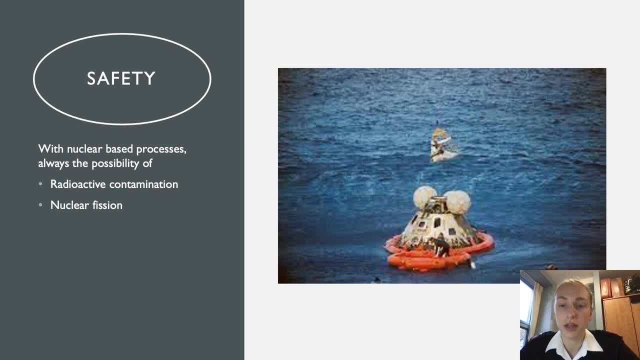 In this case, there is risk that RTG fuel leaks or an RTG fuel leak will cause an electrical conflict. In this case, there is risk that an miasma of a nuclear power plant or an RTG explodes while launching. This would create substantial lasting radioactive contamination. 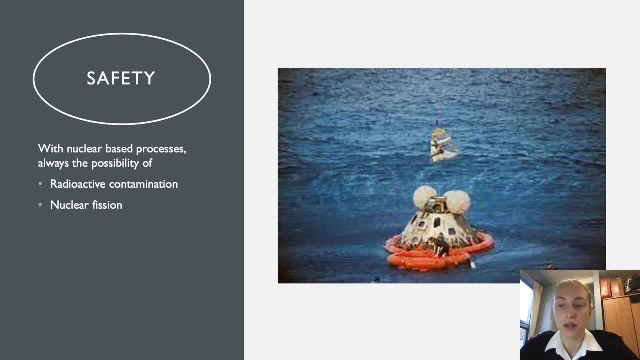 in the atmosphere, along with the possible radiation damage to all Earth and its inhabitants. There are safety measures in place to minimize these risks. For example, in the NASA mission to Saturn featuring the Cassini-Huygens probe, the RTG isotope fuel was stored inside blocks. 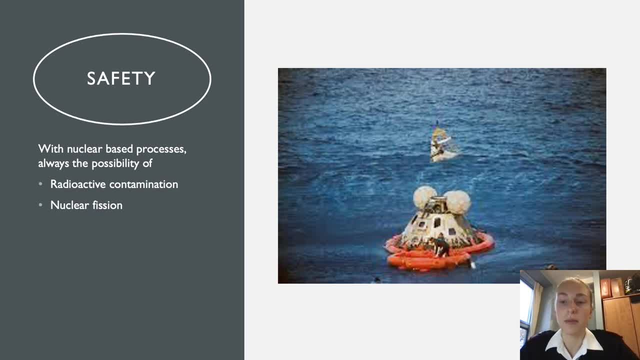 of graphite and surrounded by a layer of iridium metal to minimize the risk of accidental explosions. These graphite blocks have proven to be successful in preventing radiation contamination, as in the case of the failed Apollo 13 landing in 1970, which left its RTG in the ocean after. 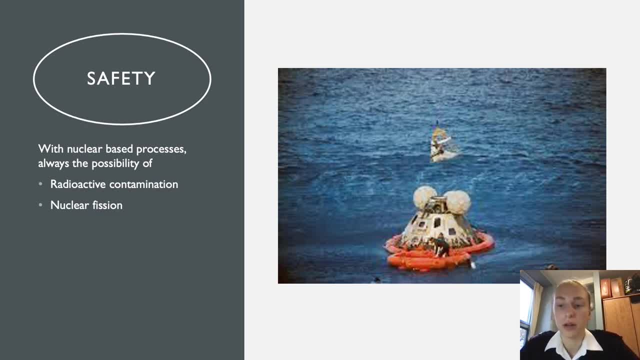 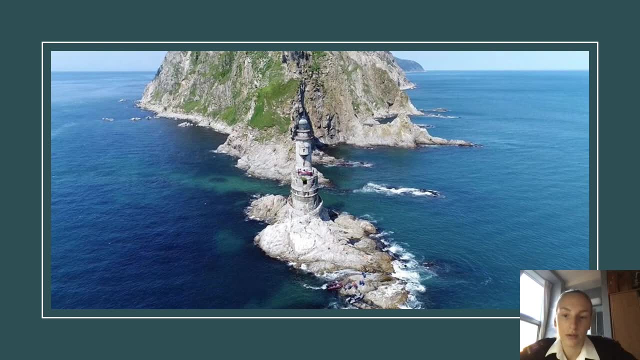 its return to Earth, but with no detectable plutonium contamination. We will now be getting into the applications of RTGs, which I think is the coolest part. So let's get started. So the Soviet Union built 1,007 RTGs to power, uncrewed lighthouses and navigation beacons. on the Soviet Arctic coast or the Arctic Circle by the late 1980s. These lighthouses were not maintained for many years after the dissolution of the Soviet Union in 1991.. Some of the RTG units disappeared during this time from either looting or by natural causes. 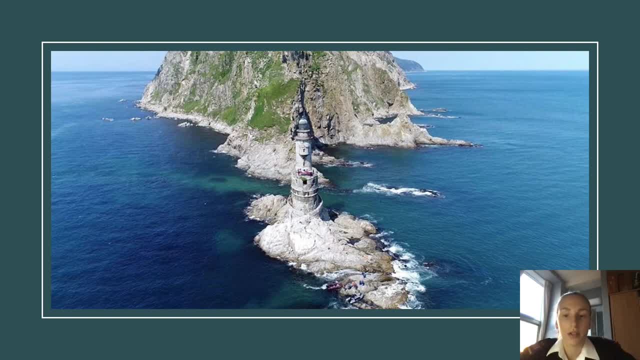 Since the dissolution of the Soviet Union, Russian and international supporters began a project to decommission the Soviet Union. The Soviet Union was the first to launch a mission to decommission these RTGs remaining in the lighthouses, and they have now all been. 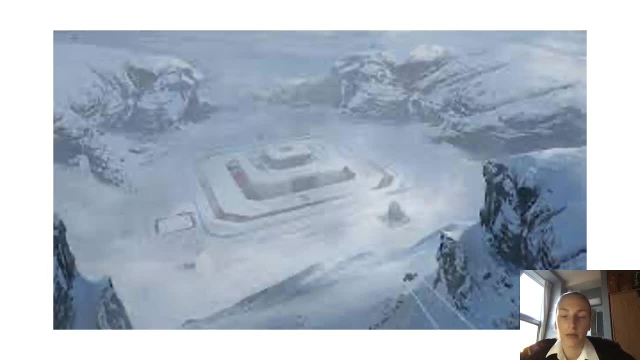 successfully removed. So pictured here is a remote base in the Arctic that is powered by an RTG. Clearly it's not getting a lot of sunlight and has probably no proximity to any major power reserves, so an RTG in this case is very useful.